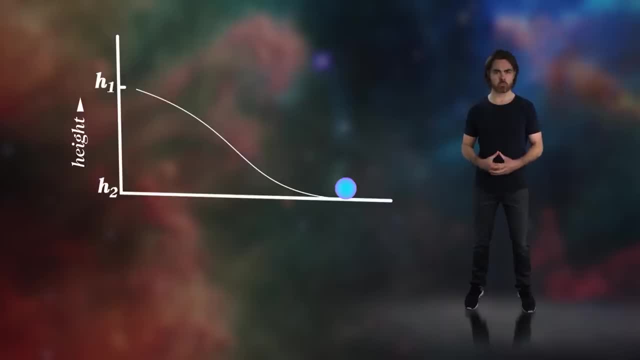 But it doesn't matter what we define to be altitude zero, the bottom of the hill, sea level, even the center of the Earth. For the equations of motion of the ball, the altitude zero point is irrelevant. It's what we call a gauge freedom or a gauge symmetry. 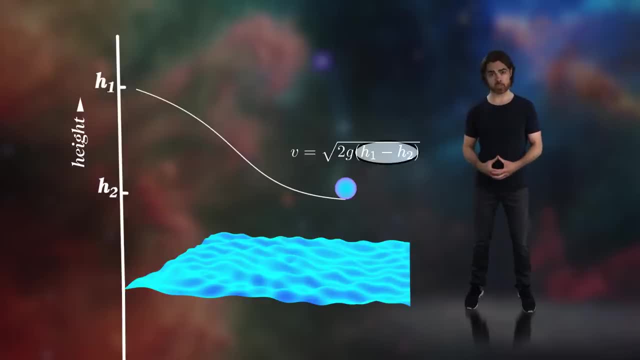 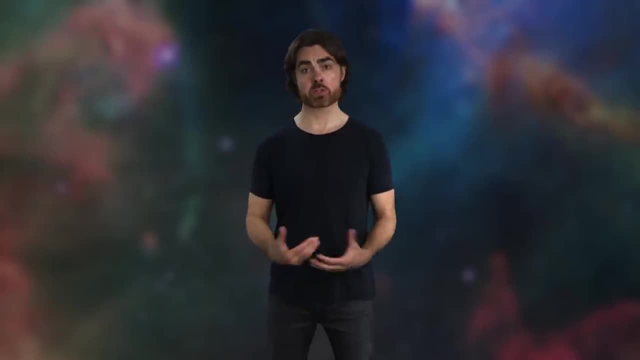 And we say that the equations of motion are invariant to that parameter. That's a pretty basic example, but it turns out that These gauge symmetries are an important feature of most of our physical theories describing the universe: Newton's laws of motion and gravity. 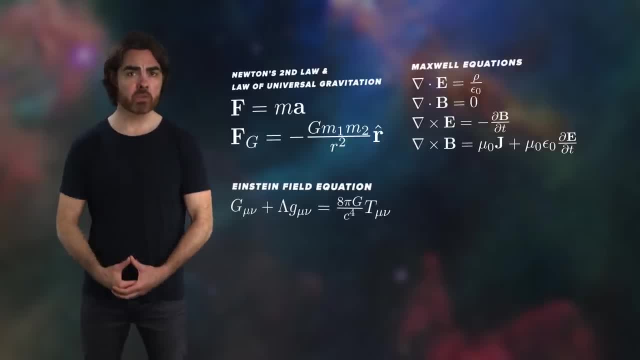 Maxwell's equations for electromagnetism, Einstein's general relativity and, of course, the standard model. We're not quite sure why this is the case, but it seems to be a trend. A theory that has these gauge symmetries is called a gauge theory. 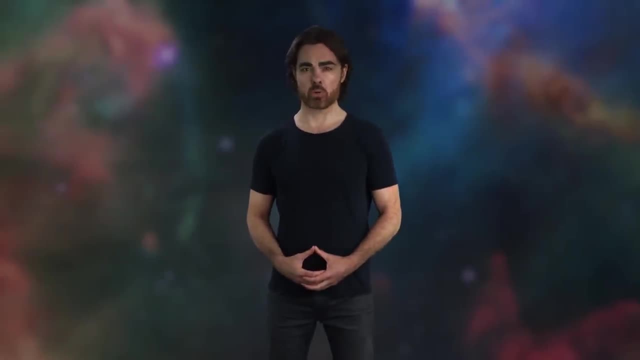 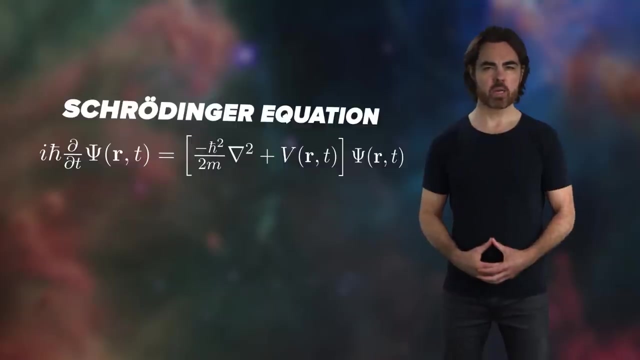 Today we're going to look at the simplest of the symmetries of the standard model. The standard model is ultimately based on quantum field theory, but we're going to use the Schrodinger equation. That's the most basic equation of motion of quantum mechanics. 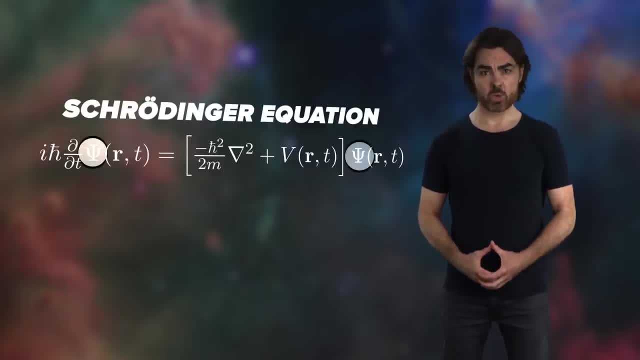 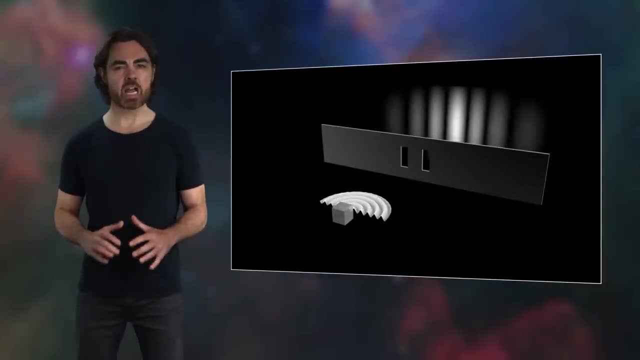 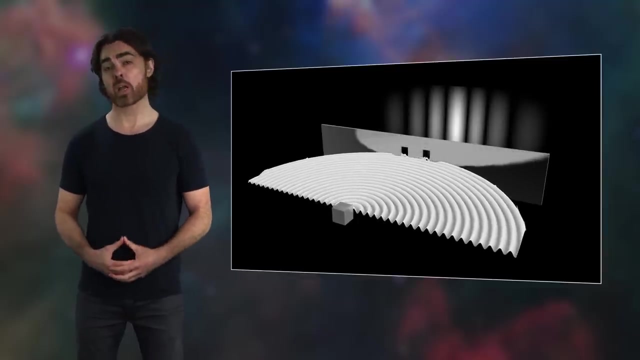 It describes the evolution of the wave function, which is the mathematical object that contains all the information about a particular physical system. We could never see the underlying wave function of, say, a particle. The best we can do is make a measurement of physical observables like position or momentum. 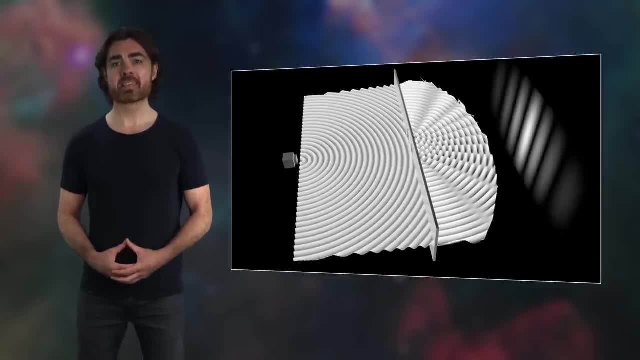 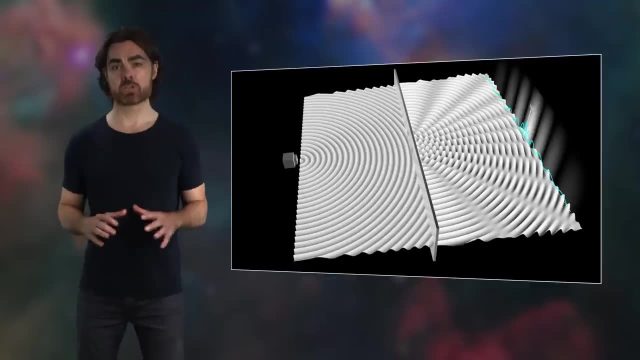 The wave function can represent different observables and it's possible to determine the distribution of possible results of measurement of those observables. In this episode, we'll be talking about the position wave function. OK, pay attention to this bit of math. 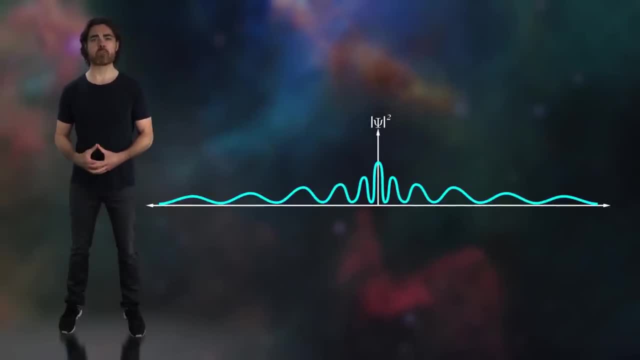 It'll be important. The square of the magnitude of this wave function tells us the probability distribution of a particle's position. The position that we observe when we look at the particle is picked randomly from that distribution. This step of squaring the wave function 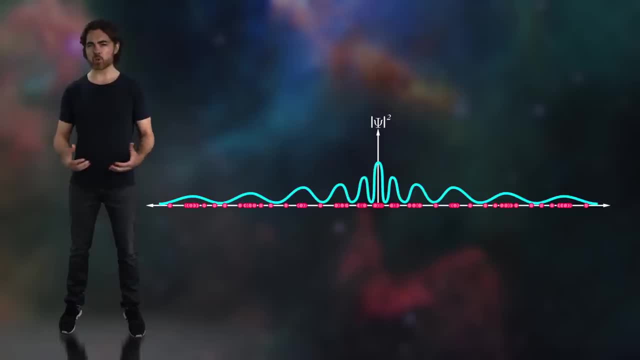 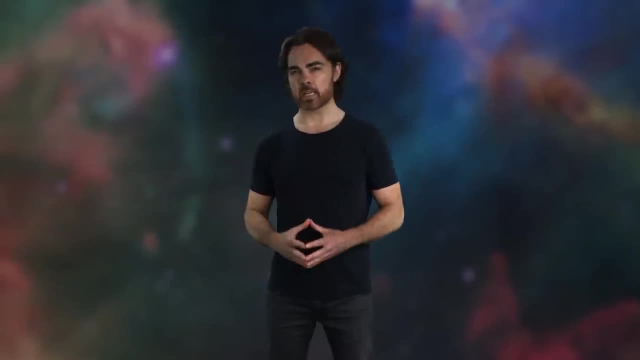 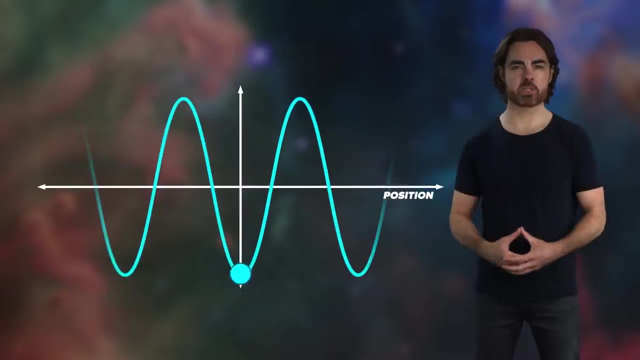 is called the Born rule, and this innocuous seeming step introduces a simple symmetry that has profound implications. Let's see what happens when we square the wave function. The wave function is an oscillation in quantum possibility, moving through space and time. It's no simple wave. 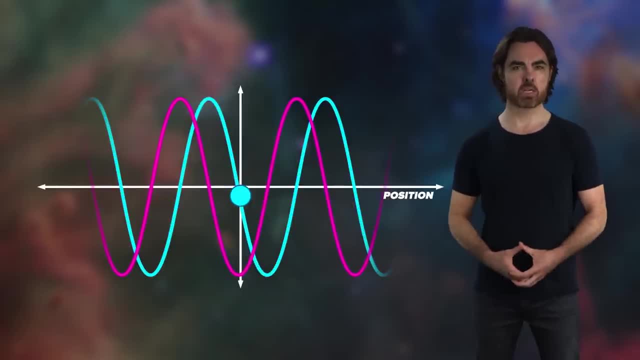 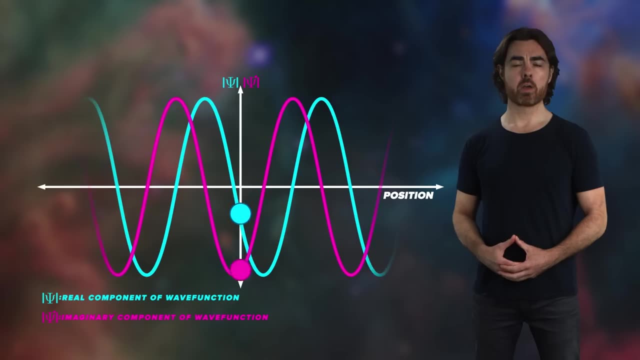 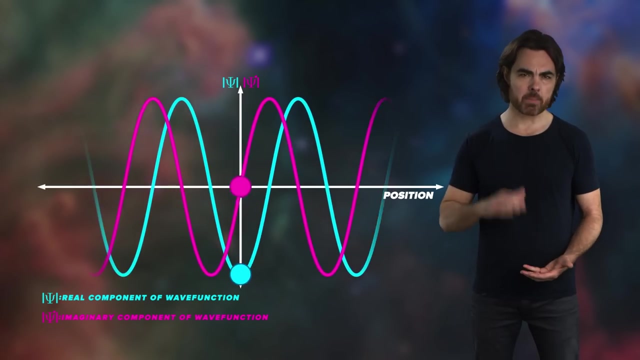 It's literally complex. in the mathematical sense, It has two components, one real and one imaginary. These two components oscillate in sync with each other, but they're offset, shifted in phase by a constant amount. Phase is just the wave's current state. 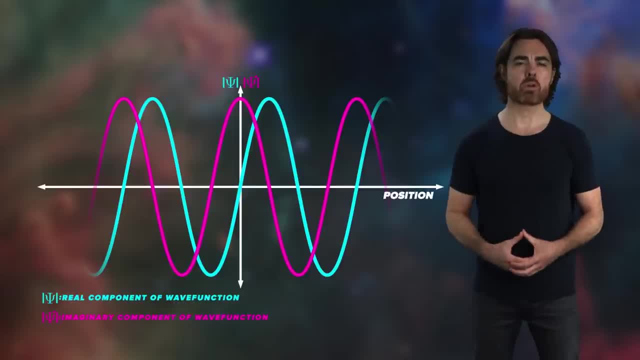 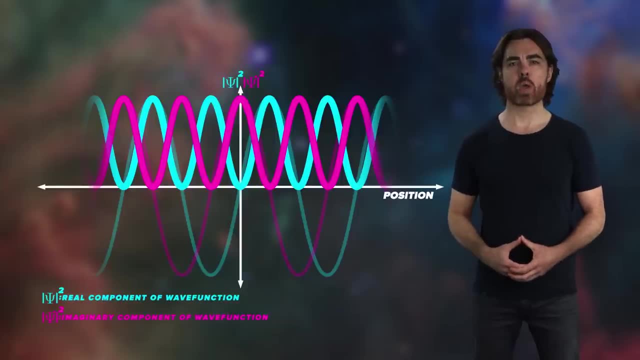 in its up-down oscillation. When we apply the Born rule, what we're doing is squaring these two waves and adding them together, But it turns out that this value doesn't depend on phase, The magnitude squared of the real and imaginary components. 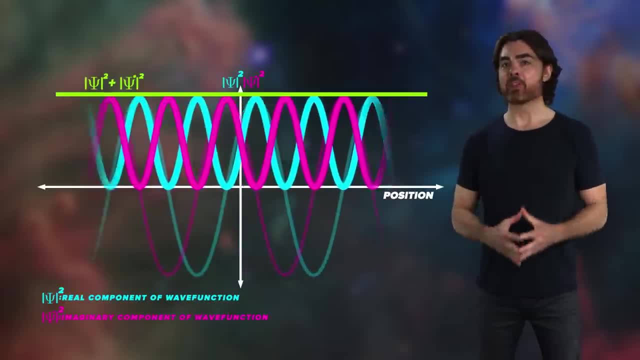 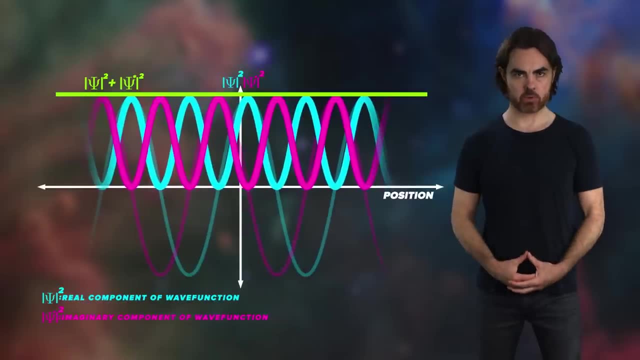 stays the same, even as those components move up and down. It's that magnitude, squared, that we can observe. It determines the particle's position. The phase itself is fundamentally unobservable. You can shift phase by any amount and you wouldn't change the resulting position. 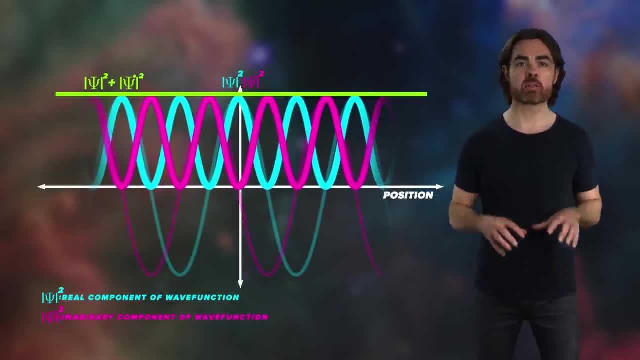 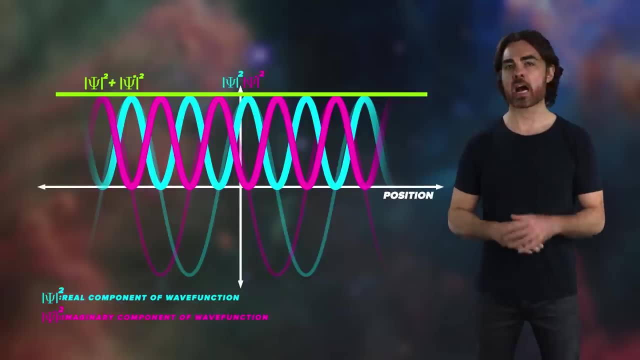 of the particle. as long as you do the same shift to both the real and imaginary components, In fact, as long as you make the same shift across the entire wave function, all observables are unchanged. We call this sort of transformation a global phase. 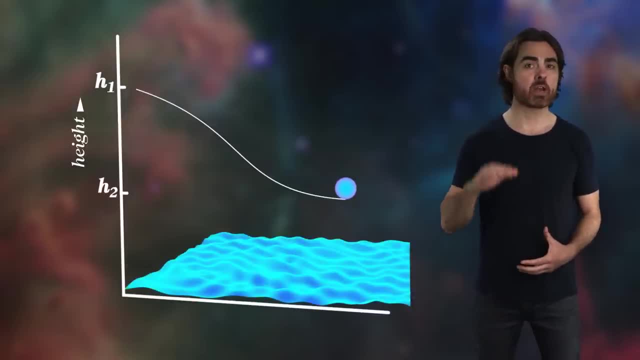 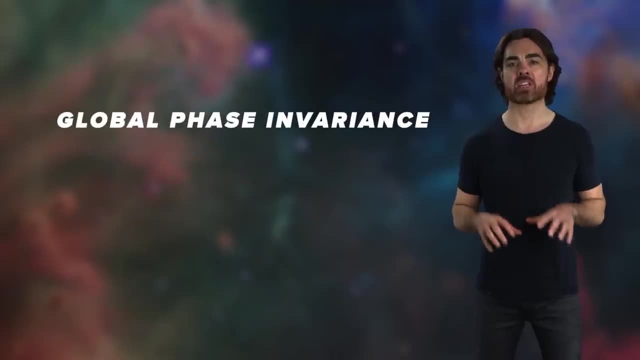 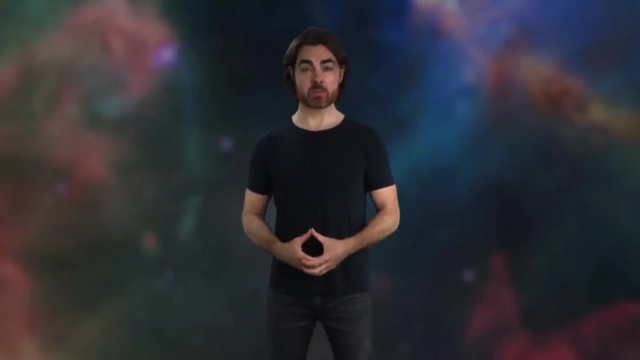 shift and it's analogous to transforming our altitude 0 point up or down by the same amount everywhere. The equations of quantum mechanics have what we call global phase invariance. Global phase is a gauge symmetry of the system. Let's push a little further to see how far this symmetry goes. 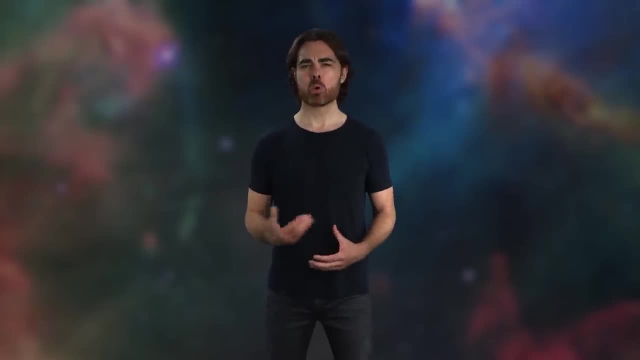 This time we'll shift the phase by different amounts at different locations, while still keeping the real and imaginary shifts the same at each location. This position-dependent phase shift is called a local phase shift instead of a global phase shift. We'll try this because, well, we already. 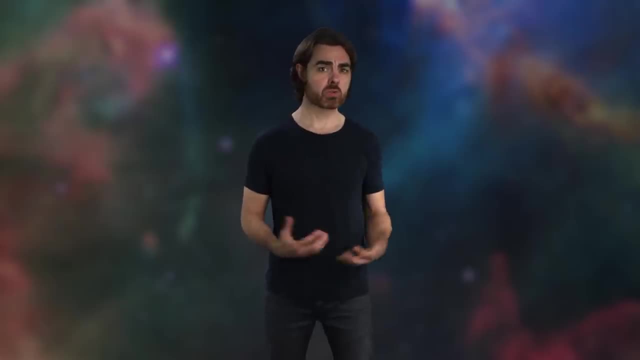 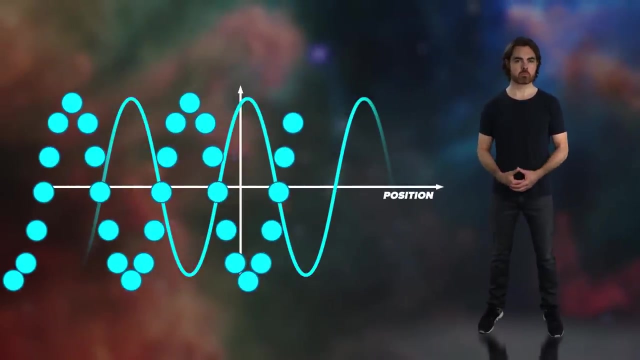 know that the magnitude squared of the wave function should still stay the same under local phase shifts. Let's see what this would look like. A global phase shift looks like this, where all points move by the same amount. However, if we do a local phase shift, say only this point here. 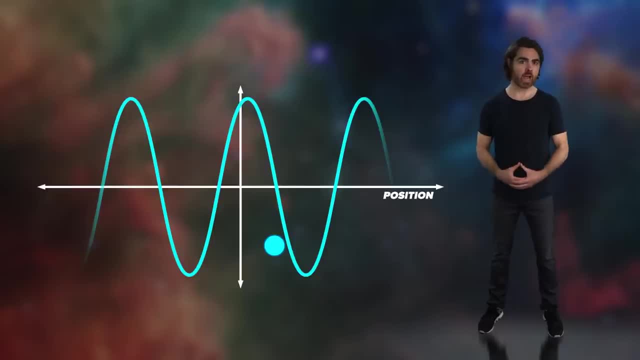 only that location changes, as if it were part of the shifted wave, making a discontinuous spike. If you allow this sort of local phase shift, you can change each point in a different way and really mess up the wave function. That shouldn't change our probabilities. 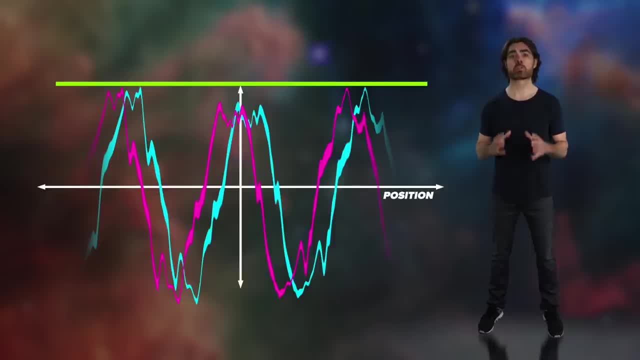 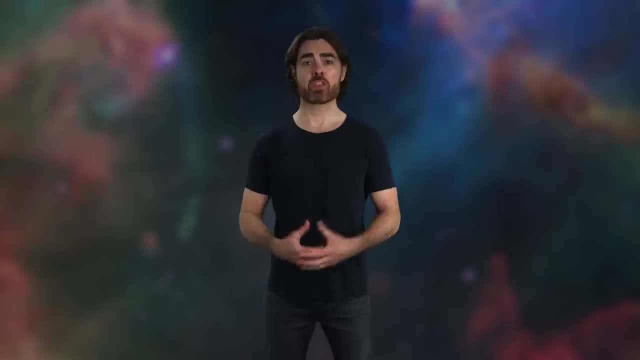 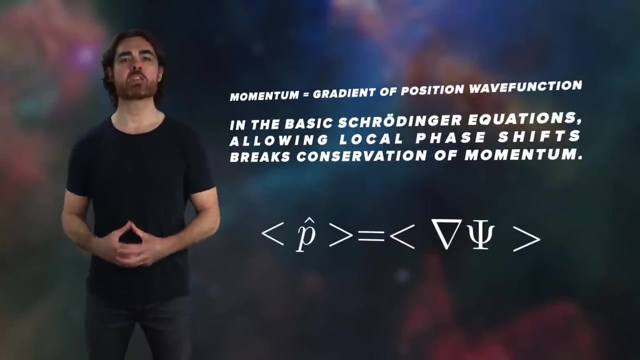 for the positions of the particles. but what about observables besides position According to the basic Schrodinger equation? we just ruined everything. Among other things, messing with local phase really screws up our prediction for the particle's momentum. See. momentum is related to the average steepness. 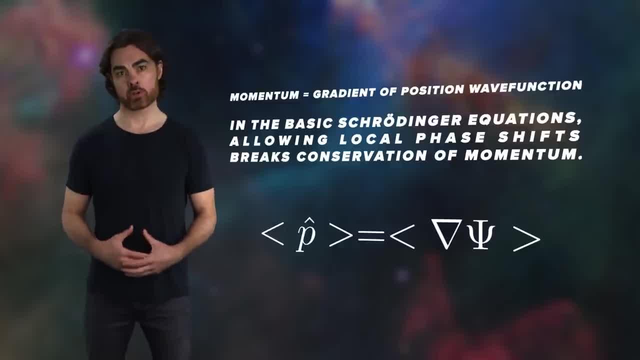 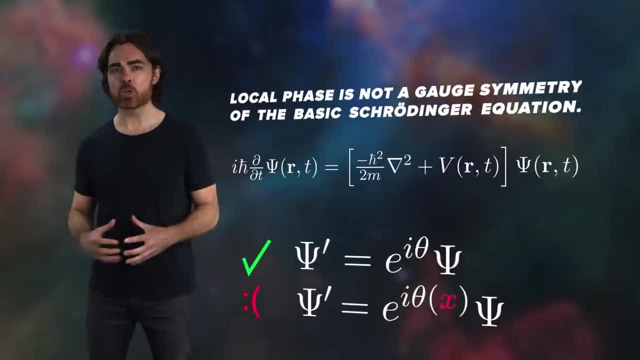 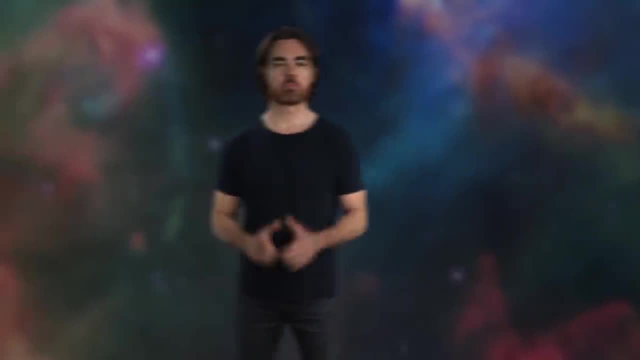 of the wave function. Change the shape of that wave function with local phase shifts and you actually break conservation of momentum. Local phase is not a gauge symmetry of the basic Schrodinger equation. OK, that was a bust. I guess we're done here. 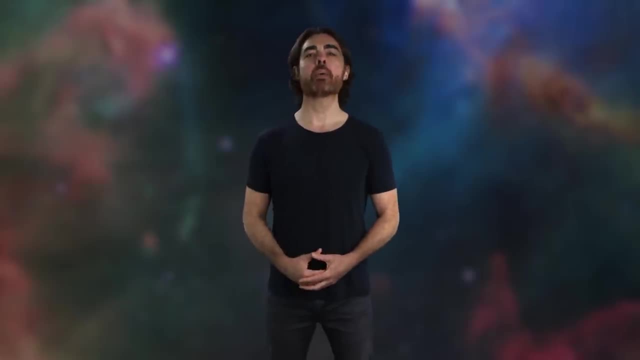 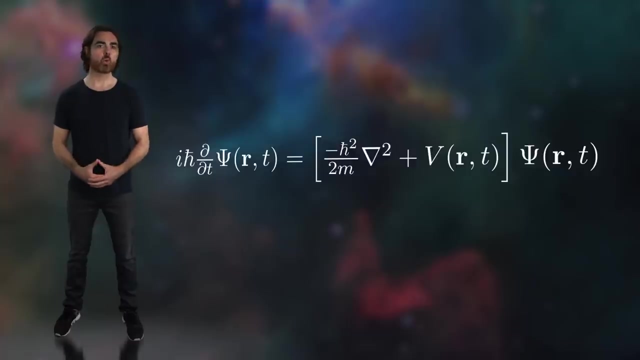 All right, wait just a second, Just for funsies. maybe we can change the Schrodinger equation to find a version that really is invariant to local phase shifts. To do that we need to alter the part of the Schrodinger equation. 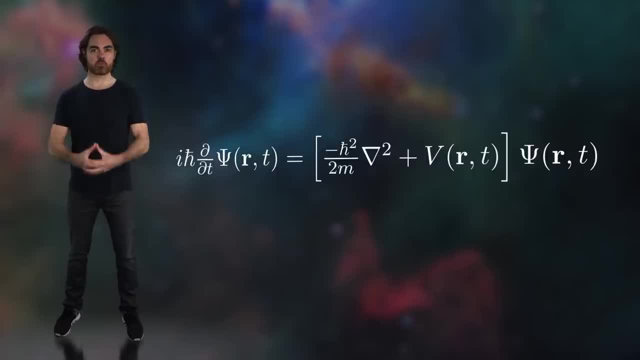 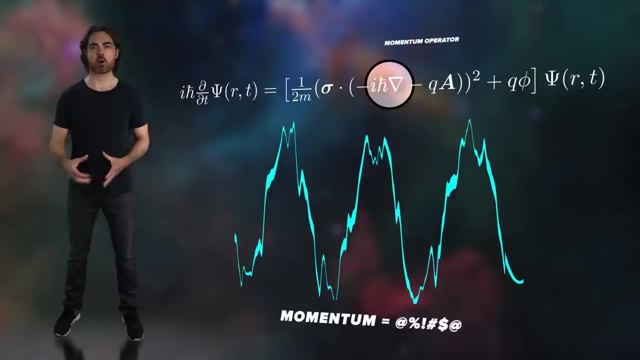 that gives us the momentum of our particle, the momentum operator. After all, momentum is what got screwed up. It turns out that we can add a mathematical term to the momentum operator that's specially designed to undo any mess we make to the phase of the wave function. 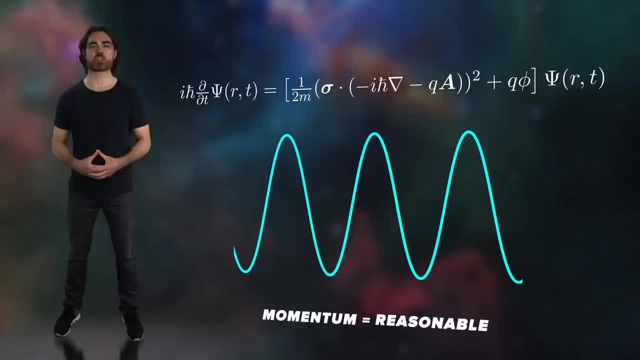 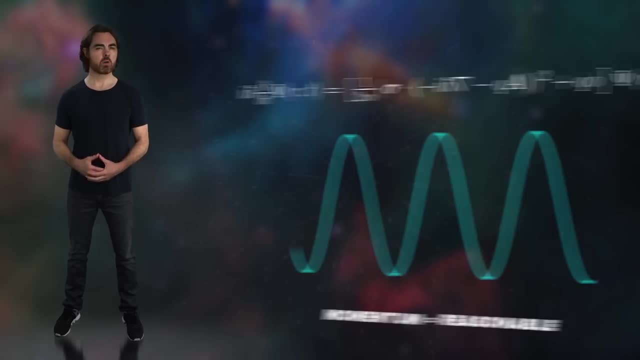 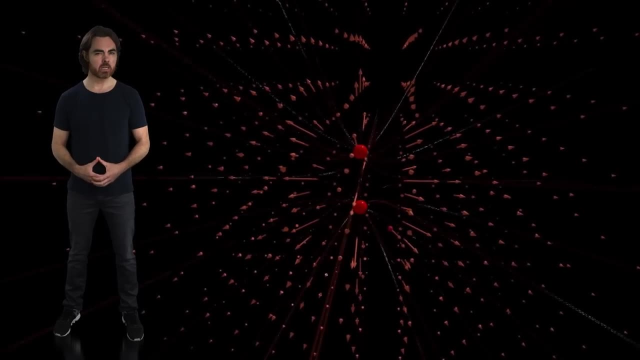 If we tune this term correctly, it absorbs any local changes we make to the phase. And what is that extra term? Well, it's something we call a vector potential. I won't go into that right now. but the important and absolutely bizarre thing about this mathematical entity- 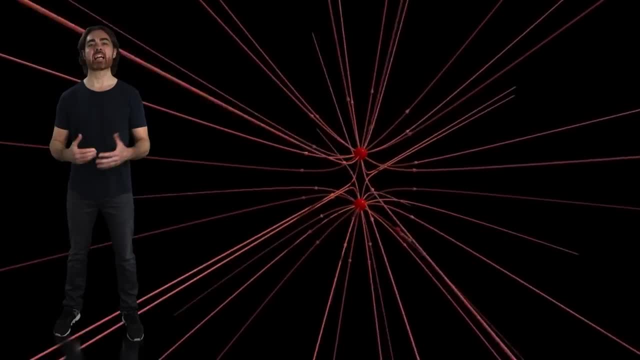 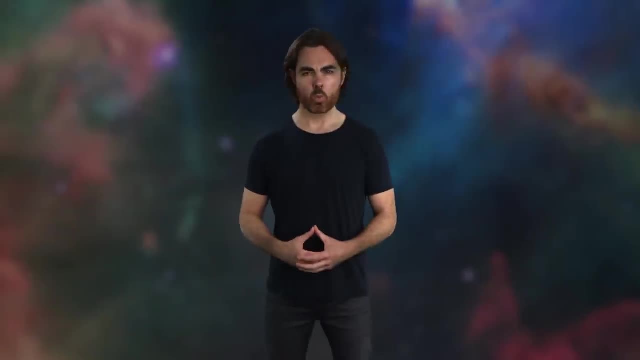 is that it looks like something very strange, OK, OK, Does that sound very familiar? It looks exactly like the type of vector potential that you would have in the presence of an electromagnetic field. So we've discovered that the only way for particles to have local phase invariance is for us. 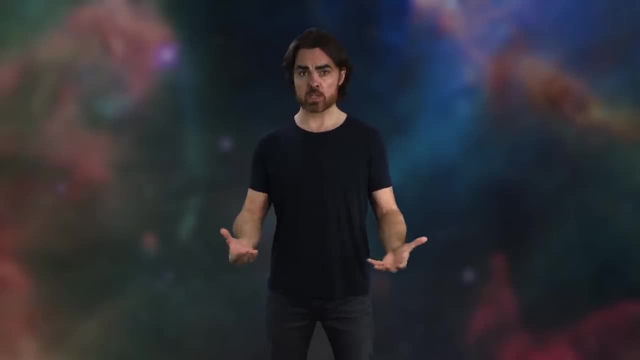 to introduce a new fundamental field that pervades all of space. And it turns out that field already exists And it's the electromagnetic field. This is totally crazy. We just rediscovered electromagnetism by insisting on a gauge shift symmetry that we had no right to expect. 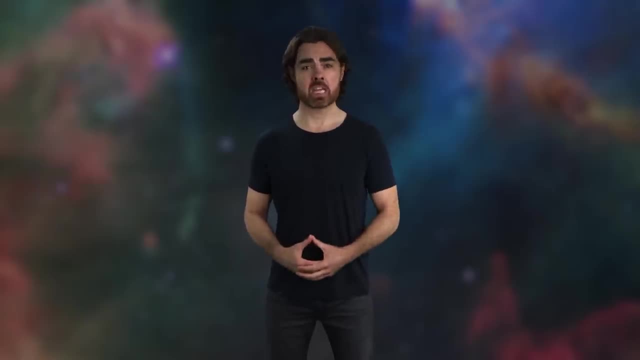 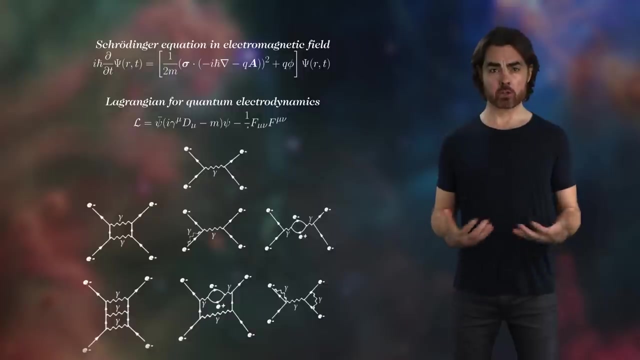 to exist in the first place. But we didn't just rediscover the EM field, We learned a ton about it. By discovering how it fits into the Schrodinger equation, we've unlocked its quantum behavior And now we know how it interacts with particles of matter. 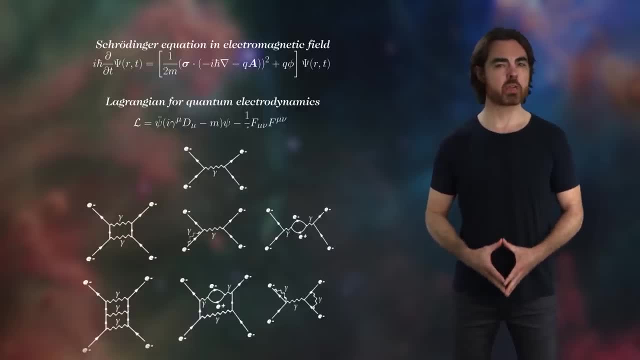 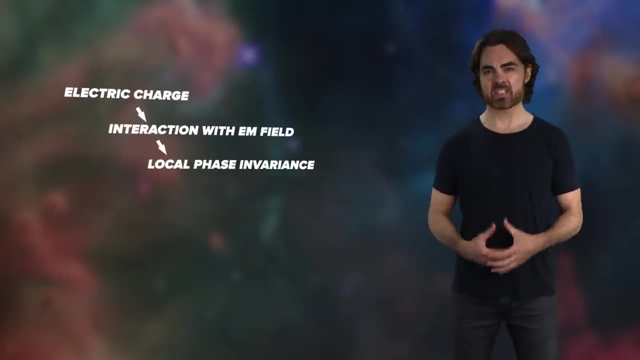 to give them this symmetry. We also learned about the origin of electric charge, which we now see as a coupling term. Any particle that has this kind of charge will interact with and be affected by the electromagnetic field and be granted local phase invariance. 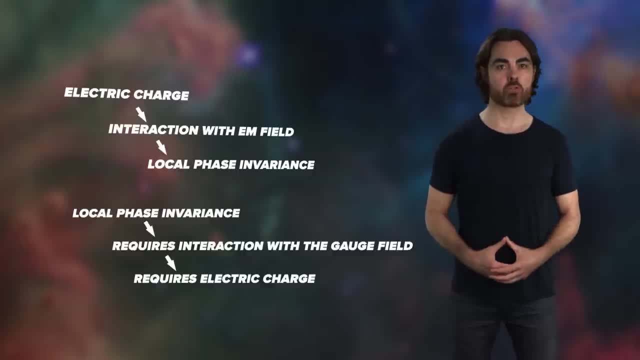 But the reverse is also true. In order to have this particular type of local phase invariance, particles must possess electric charge. By the way, applying Noether's theorem tells us there is a conserved quantity associated with any symmetry. In this case, the symmetry is local phase invariance. 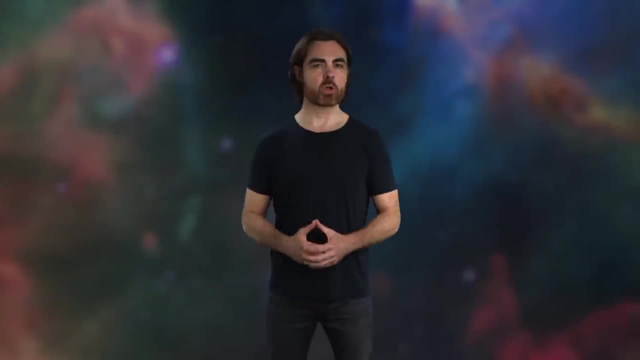 and the conserved quantity is electric charge. At this point we only need a couple of extra steps to produce the full description of electromagnetism in the quantum world, quantum electrodynamics or QED. First we need to upgrade the Schrodinger equation. 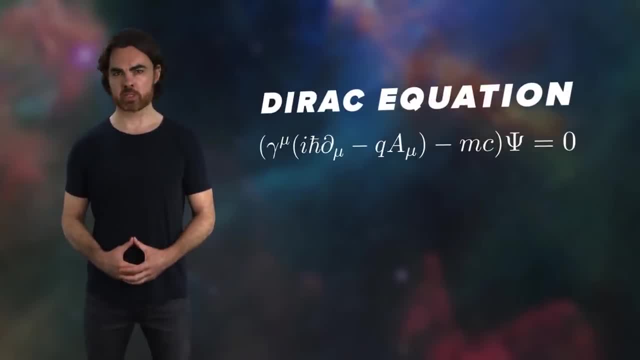 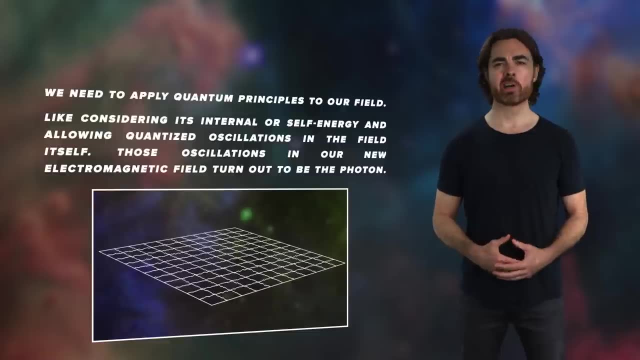 to the Dirac equation, so it works with Einstein's special relativity And we talked about that in this episode. Then we need to apply quantum principles to our field, like considering its internal or self-energy and allowing quantized oscillations in the field. 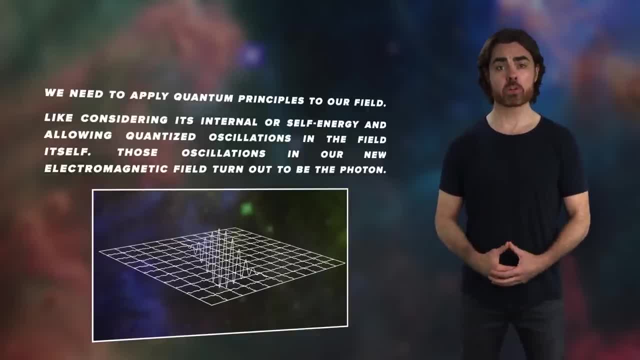 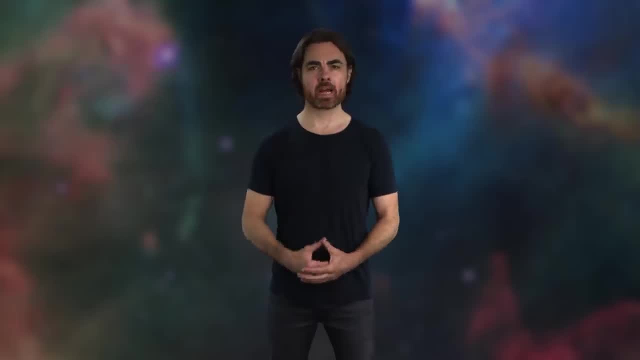 itself, Those oscillations in our new field and our electromagnetic field turn out to be the photon. But what about all those fundamental particles without electric charge, neutral particles like neutrinos? To understand those we'll need to go beyond the Schrodinger equation and to explore new gauge. 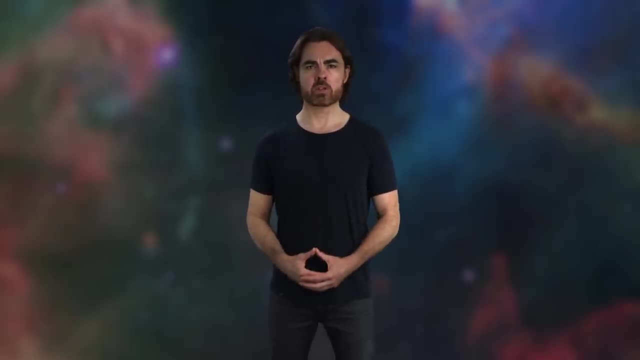 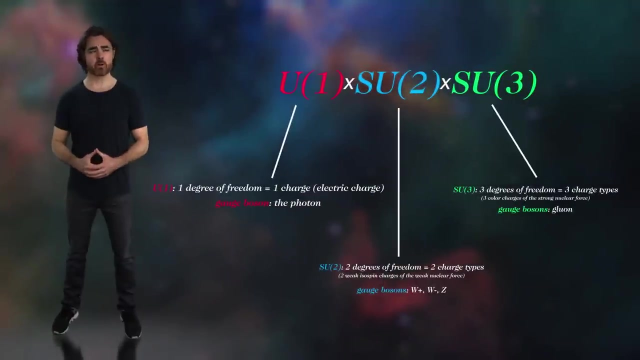 symmetries. It turns out that local phase invariance is just the simplest of the largest suite of gauge symmetries of the standard model. Those symmetries are obtusely named U1, Su2, and Su3. And they predict the fields that give rise. 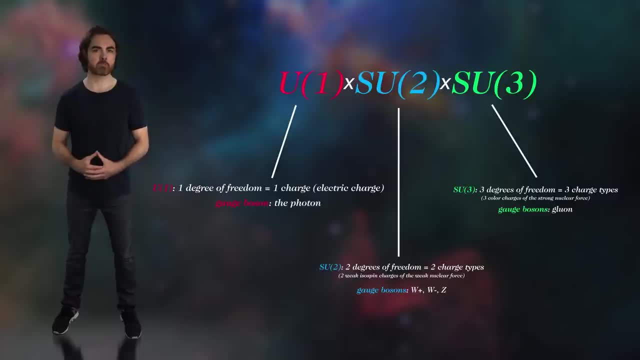 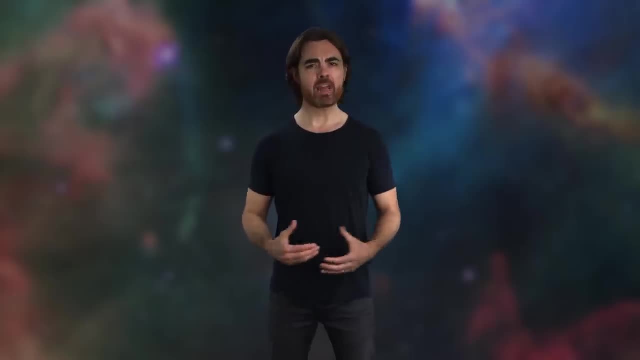 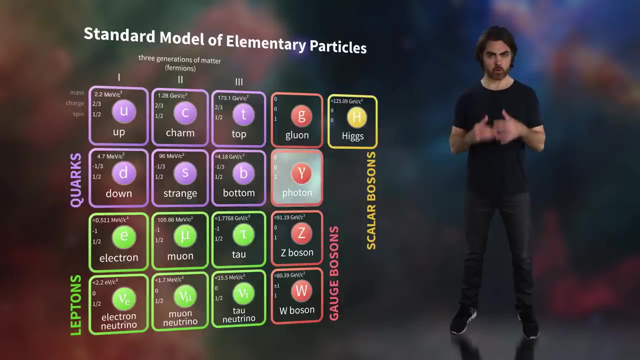 to electromagnetism, the weak and the strong nuclear forces respectively. The fields that arise from these gauge symmetries are called gauge fields, And they all have their associated oscillations, their associated particles. These are the gauge bosons, the photon for electromagnetism. 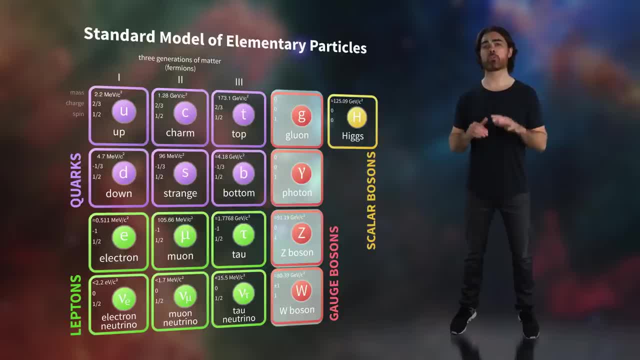 the W and Z bosons for the weak interaction and the gluon for the strong interaction. Together they govern the interactions of the matter particles of the standard model And we'll come back to that in future episodes. Perhaps the greatest mystery here. 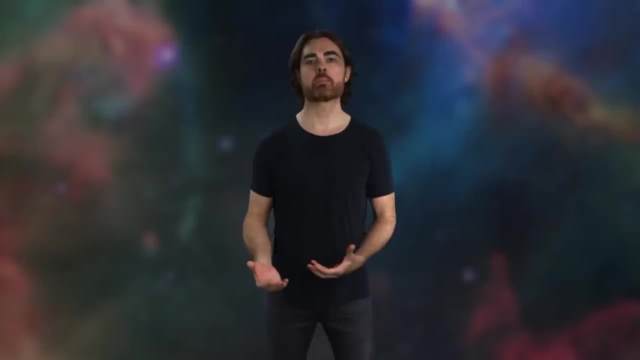 is not the nature of the quantum fields, nor the connection between symmetry and the fundamental forces. Perhaps it's the fact that by pure exploration of mathematics, delving many layers of abstraction deeper than our capacity for intuition, we are led to true discoveries about physical reality. 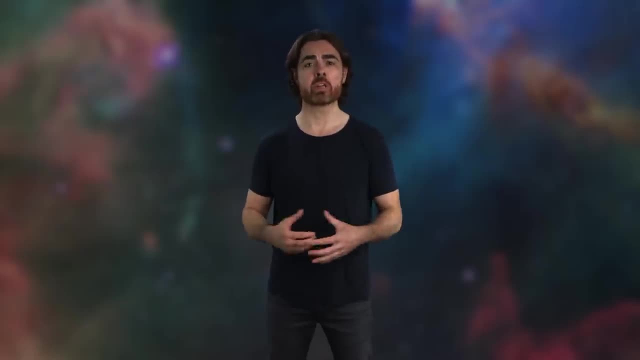 And, following those mathematical labyrinths, reveals physical theory with stunning predictive theory. It's also the fact that there is no such thing as the standard model of particle physics. Mathematics truly seems to be the language in which the universe is written. We should be amazed that we can learn that language. 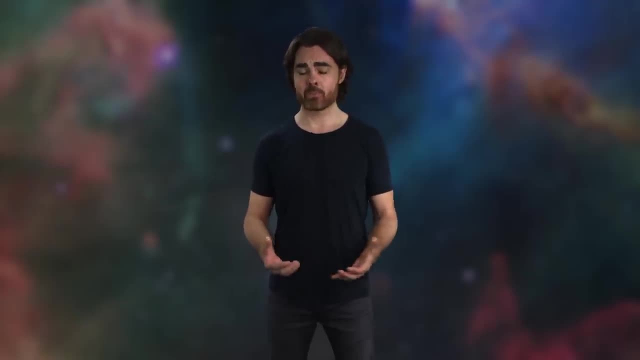 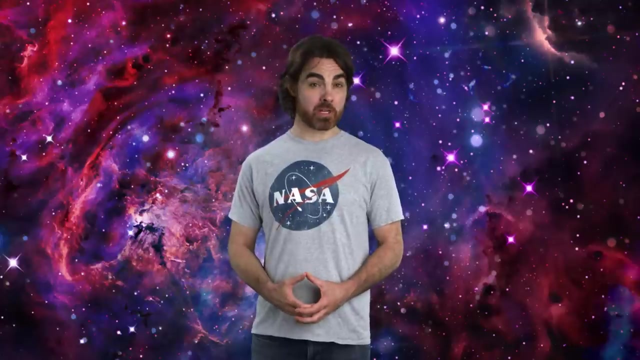 and, through it, comprehend the underlying nature of spacetime. Last time on Spacetime Journal Club, we looked at a new result potentially detecting a particle beyond the standard model, the sterile neutrino. Let's see what you had to say. 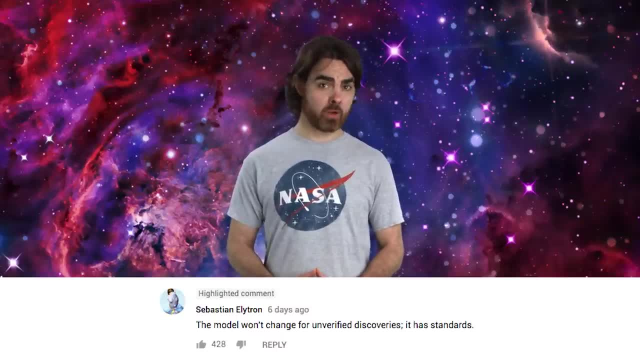 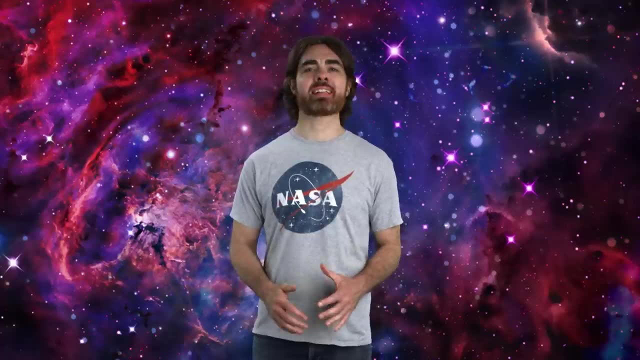 Sebastian Eletron says that the standard model won't change for unverified discovery. It's still not a discovery, It's still a new particle, But in terms of discoveries it has standards Totally agreed. And no one, not even the researchers. 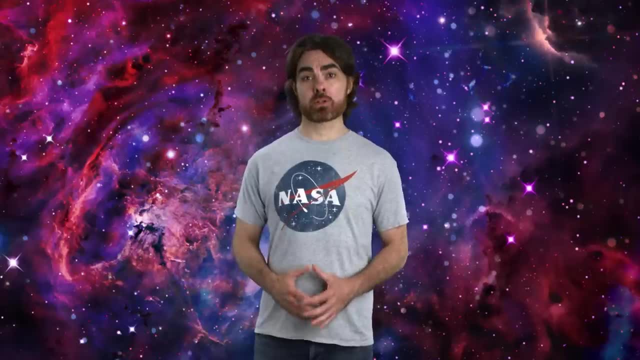 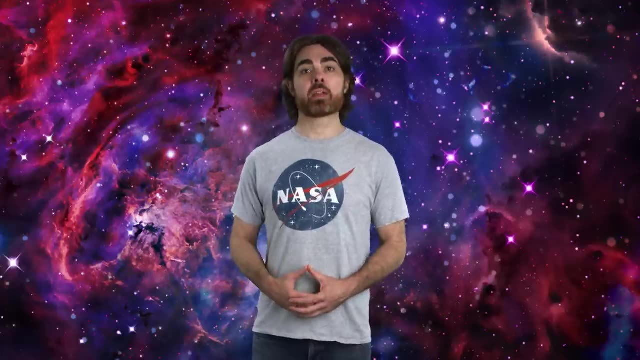 are claiming the actual discovery of this new particle. yet April put it well in a response to your comment: A 6.1 sigma level of significance doesn't mean for sure that sterile neutrinos exist. It could mean there's some other physical process. 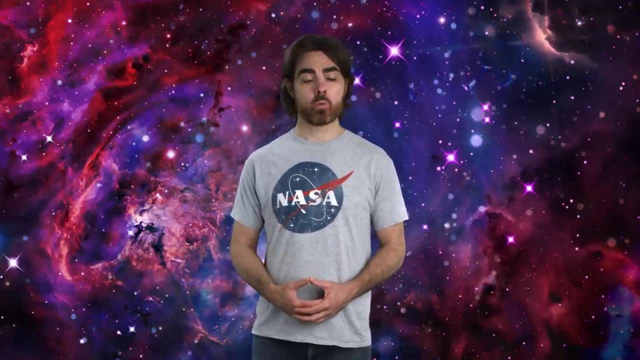 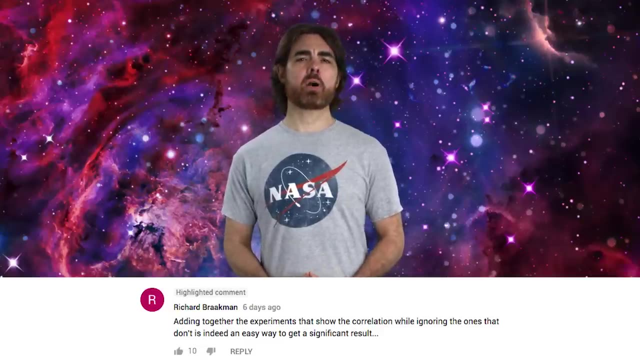 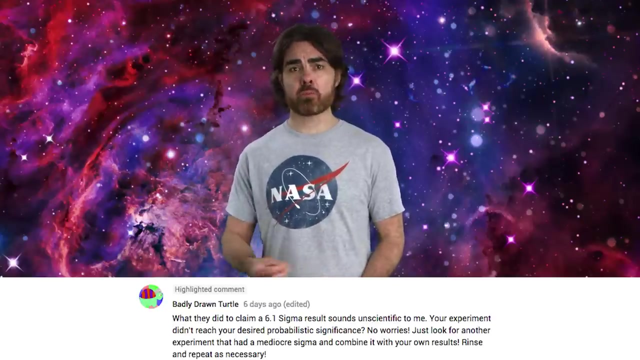 that we don't understand yet. Regardless, it'll definitely mean something happened. Will it be something interesting? Richard Brachman and Badly Drawn Turtle point out the danger of combining multiple experiments to increase the significance of your results. If you have enough experiments to choose from, you can just select from those with the highest. 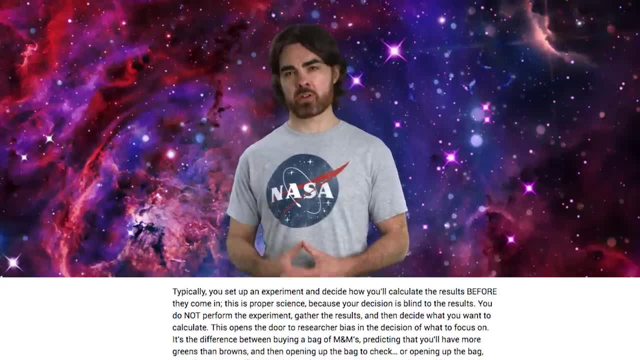 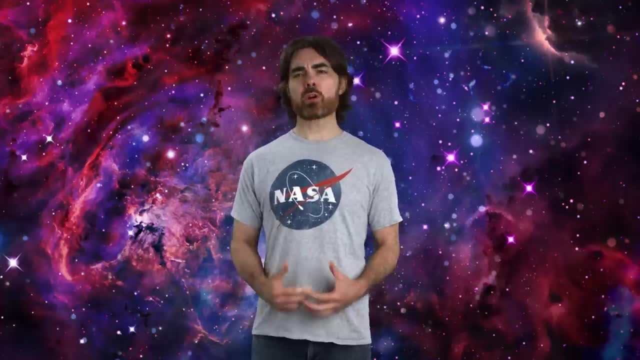 significance until it takes you over the 5-sigma significance hurdle. In the case of the MiniBoon experiment, they combined their 4.8-sigma Fermilab result with the 3.6-sigma result from the only other substantially similar experiment that has ever been performed. 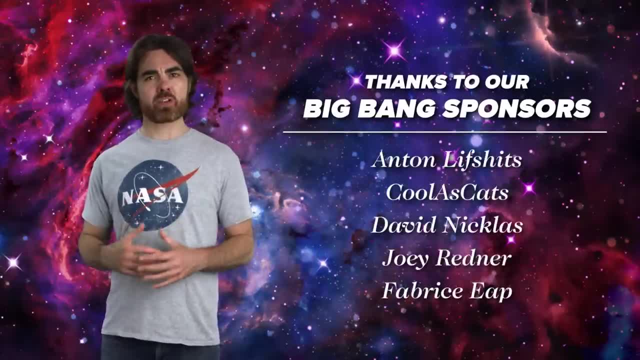 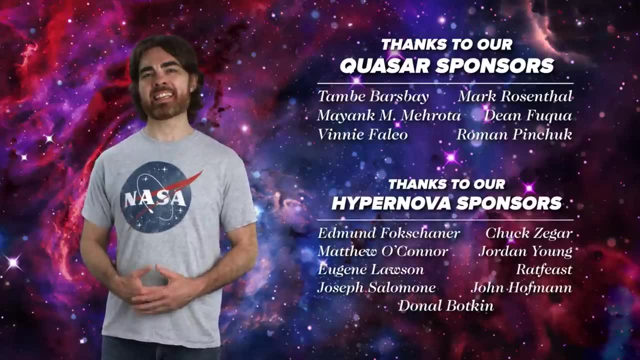 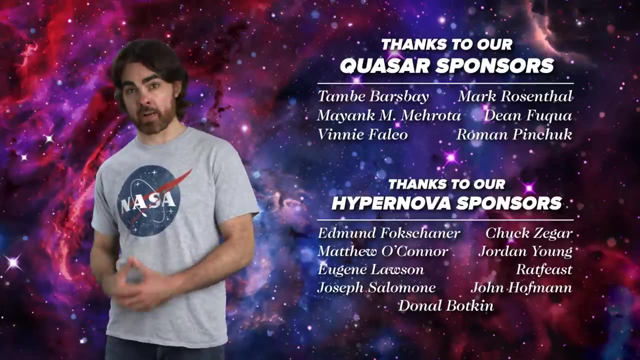 – that one at Los Alamos. So there's some justification, because there weren't any very similar experiments with lower significance. On the other hand, it seems like they didn't integrate the constraints to sterile neutrinos derived from the IceCube experiment or from the Cosmic Microwave Background Radiation.